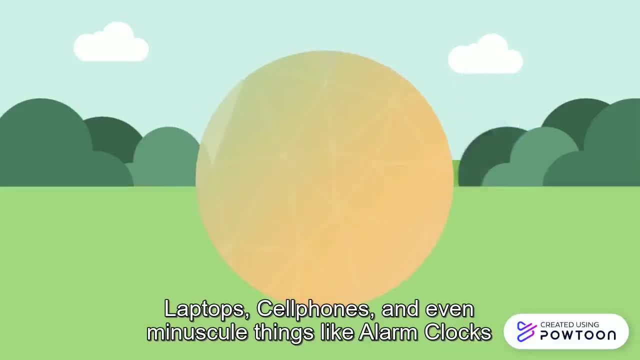 Today, we're surrounded by man-made things everywhere we go. Laptops, cell phones and even minuscule things like alarm clocks are omnipresent. But have you ever stopped to wonder what makes the design so optimal? Probably not, But if you ever did, 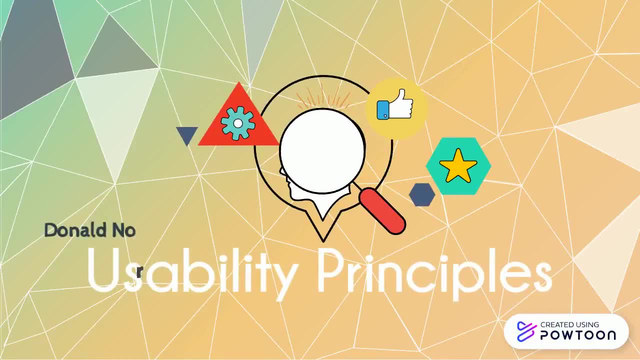 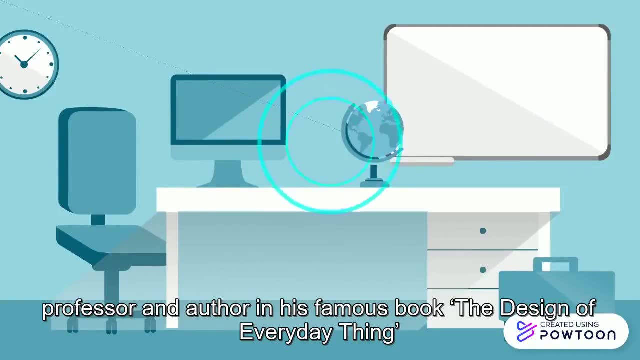 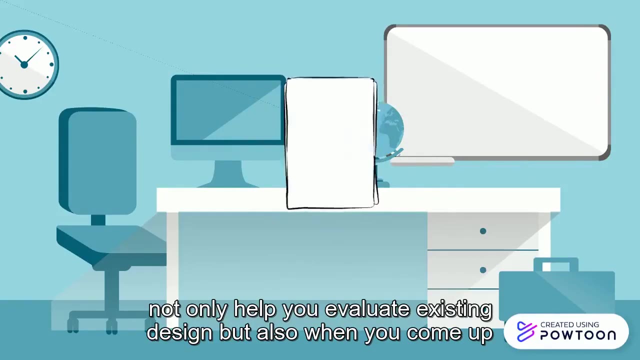 we have something that might be of help. Donald Norman, a renowned American researcher, professor and author, in his famous book The Design of Everyday Things, has laid out some principles to evaluate, as his book says, the design of everyday things, which will not only help you evaluate existing designs. 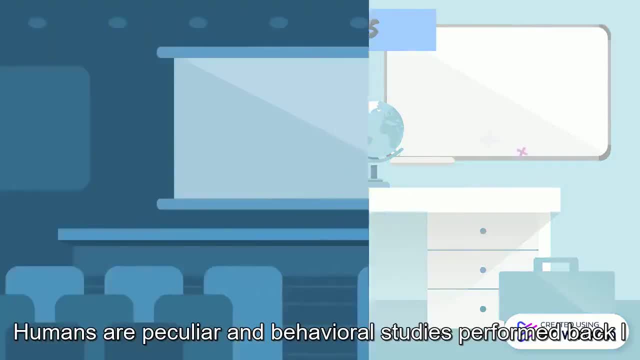 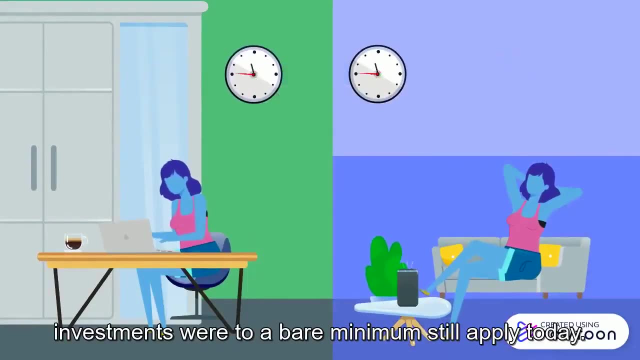 but also when you come up with your own new ideas. Humans are peculiar, and behavioral studies performed on them back Norman's principles. His book, published in 1988, when technological investments were to a bare minimum, still apply today. When used, they lay a strong. 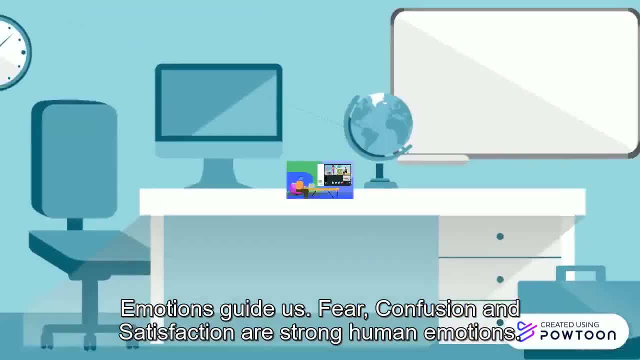 foundation for human-computer interaction. Emotions guide us. Fear, confusion and satisfaction are strong. you know. Emotions guide us. Fear, confusion and satisfaction are strong. you know. Emotions guide us. Fear, confusion and satisfaction are strong, you know. 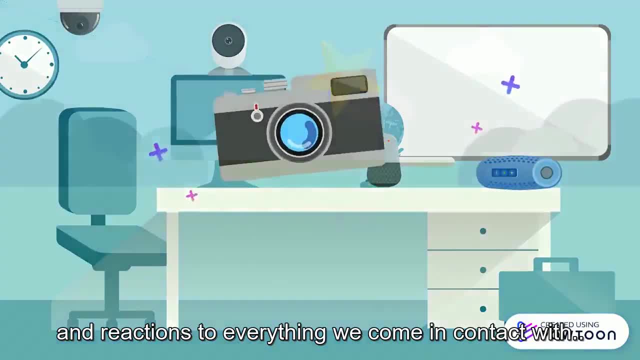 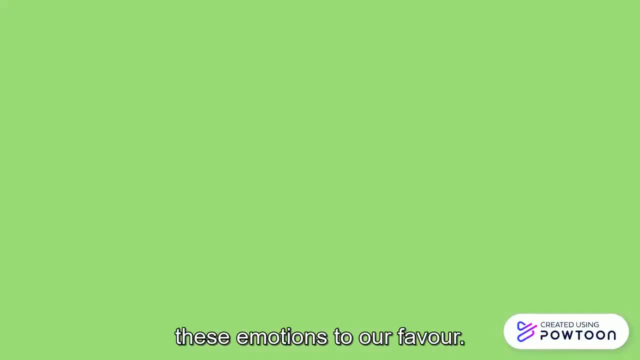 They pilot our behavior and reactions to everything we come in contact with. A happy person is more likely to solve a problem given and enjoy the time while doing so. We learn to use these emotions to our favor, Giving only the necessary piece of the puzzle. 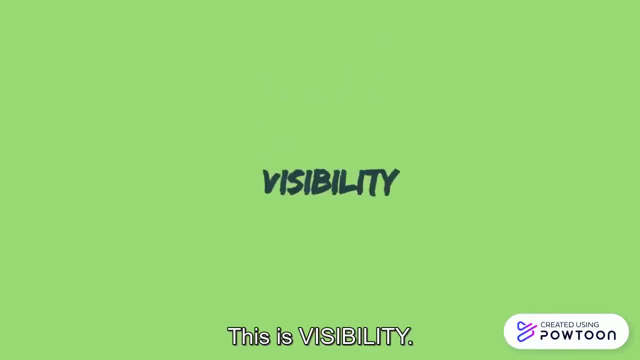 in storytelling piques user engagement and interest. This is visibility. It focuses on the principle that the more visible an item is, the more likely users will know about them and use them. Login screen needs information about login in or sign in up, but cluttering with other information is wrong. 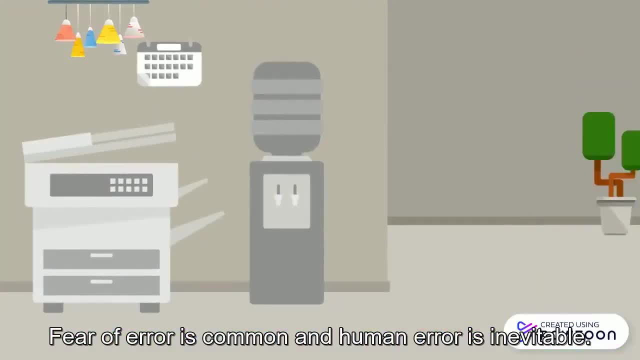 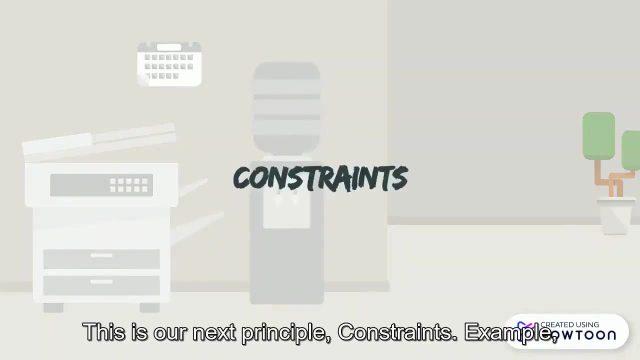 Login screen needs information about login in or sign in up, but cluttering with other information is wrong. Fear of error is common and human error is inevitable. Limiting the interaction to an interface and any possibility to making an error will help. This is our next principle: constraints An online form that does not allow users. 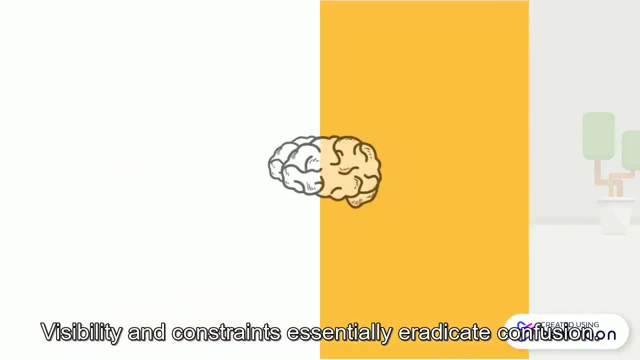 to enter letters into a phone number field. While visibility and constraints essentially eradicate confusion, the control and effect mechanism engraved in a human brain, when unchecked, can also lead to confusion. This is mapping The idea that, in a good design, the controls for something will closely resemble their effect. The idea that, in a good design, the controls for something will closely resemble their effect.